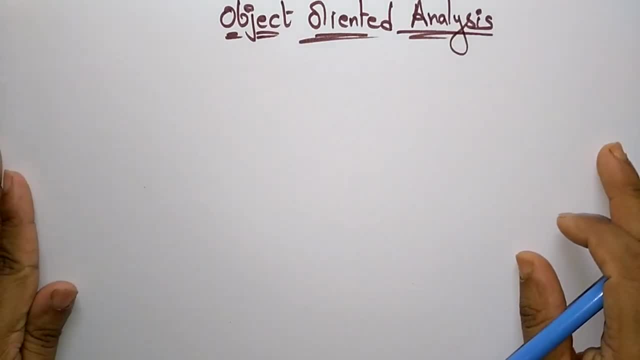 Hi students, coming to the next topic, that is, the object oriented analysis. So in this coming videos we will discuss about object oriented analysis, object oriented design and object oriented modeling. So if you want to develop any system, means, any product, you need to analyze, design and model the system. Now, first let us see what is this analyzing object oriented analysis? 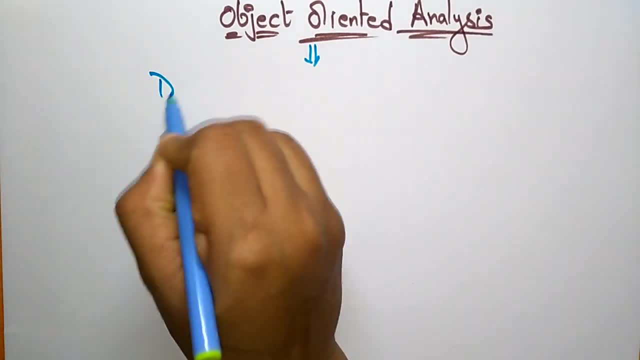 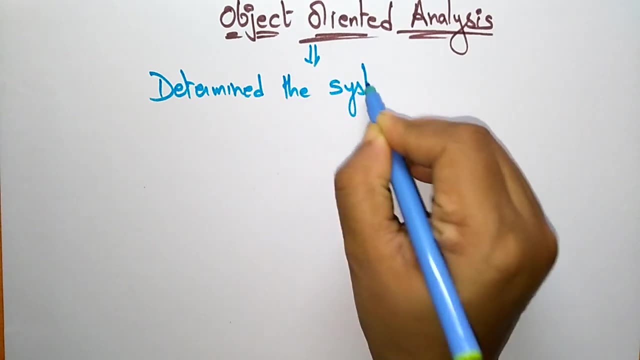 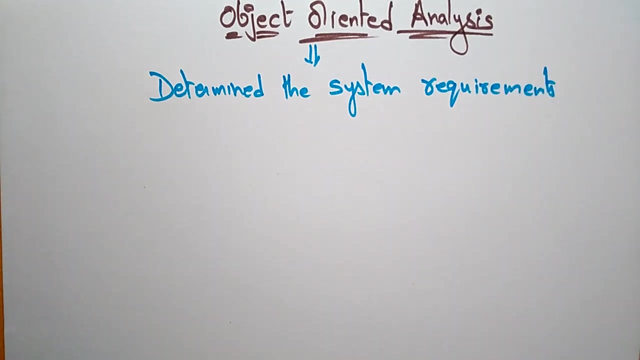 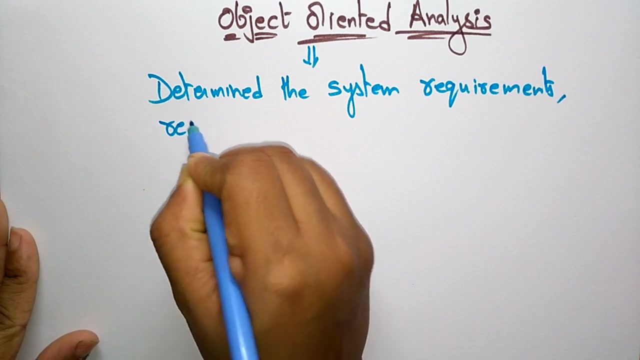 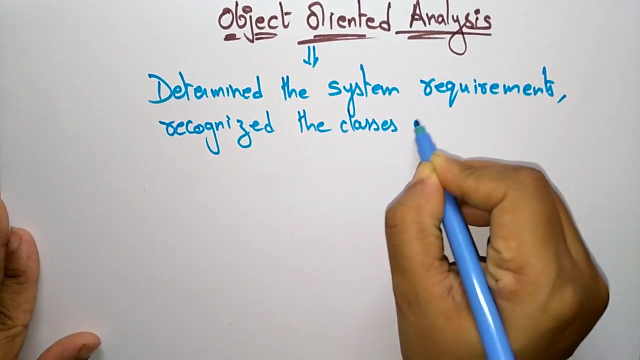 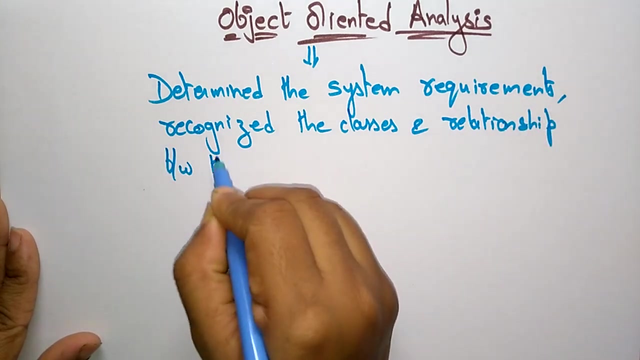 So this object oriented analysis determined the. it determined the system requirements, determined the system requirements. So, whatever the requirements that the user wants, means what the outlook of the system that requirements and recognize the classes, recognized the classes And relationships between the classes, relationship between the classes. that is called object oriented analysis. The object oriented analysis is going to determine the system requirements and it is going to recognize the classes and the relationship between those classes. The main purpose of object oriented analysis is the main purpose. 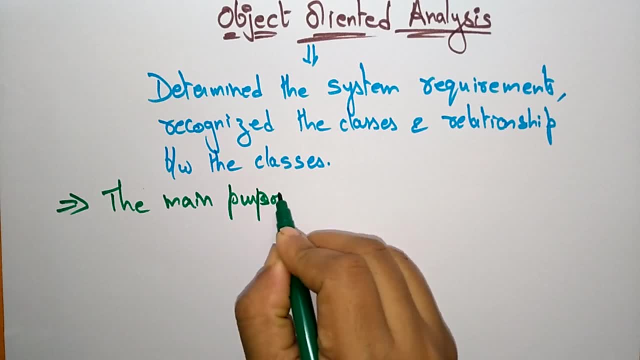 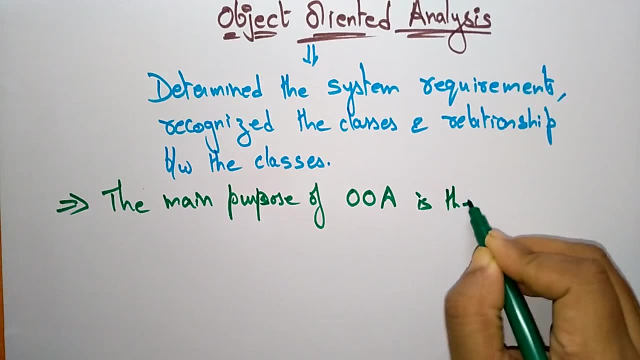 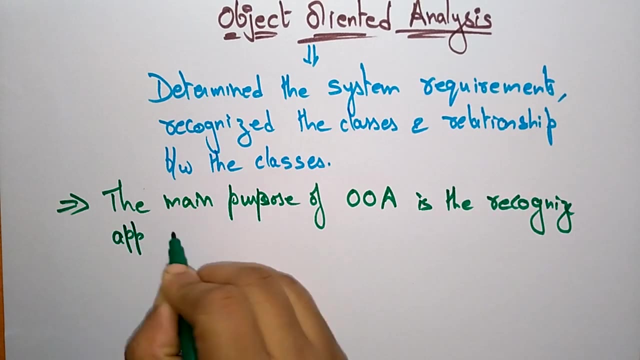 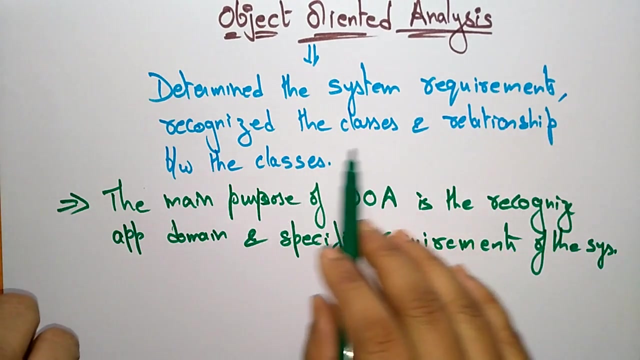 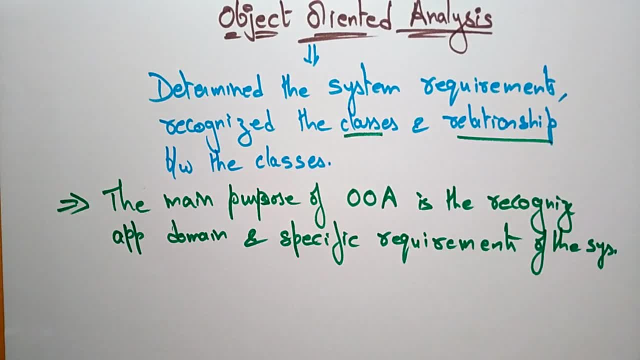 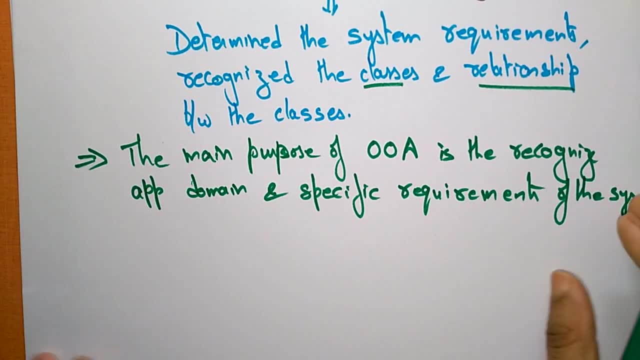 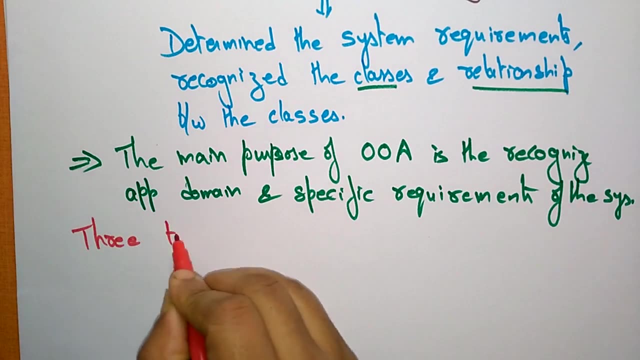 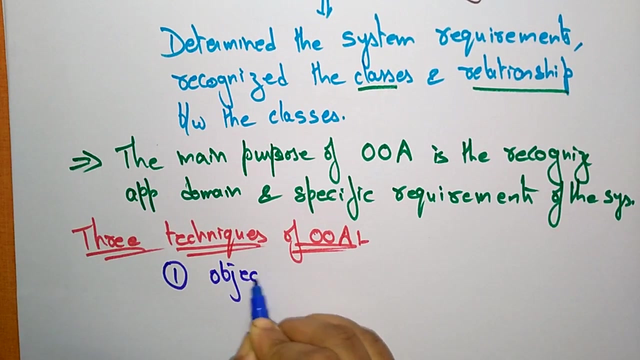 logical structure is nothing but classes and relationships. So that is the main purpose of object oriented analysis. Now let us see the techniques of object oriented analysis. Mainly there are three techniques, three techniques of object oriented analysis. so in the object oriented analysis you came across three techniques. the one is object modeling, object 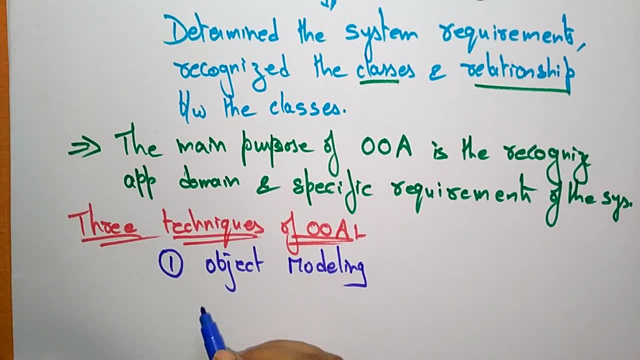 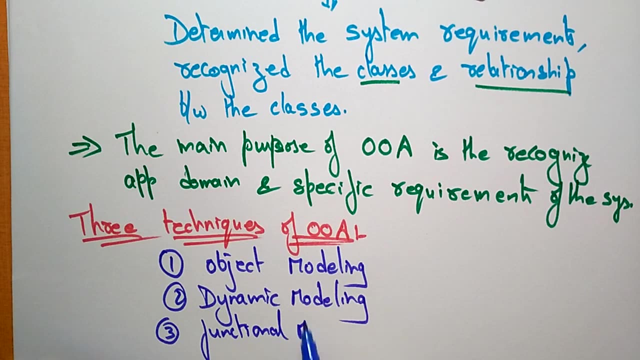 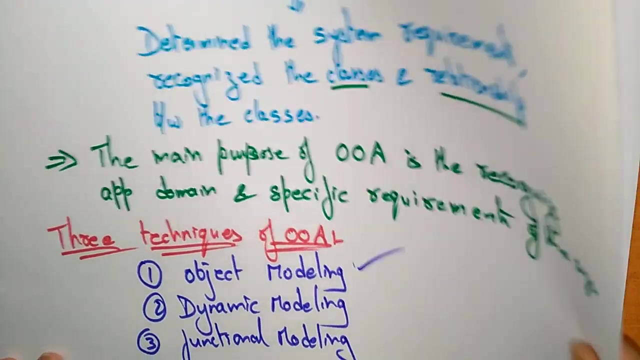 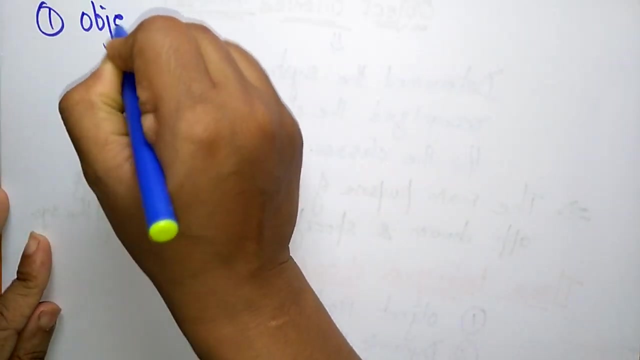 modeling, and the second one is dynamic modeling- dynamic modeling. and the third one is function modeling- functional modeling. so these are the three techniques of object oriented analysis. now let us see what is this object modeling. let me explain about object modeling. let me explain about object modeling. object modeling: so what is the name indicating we are going to model the object? so what are the? 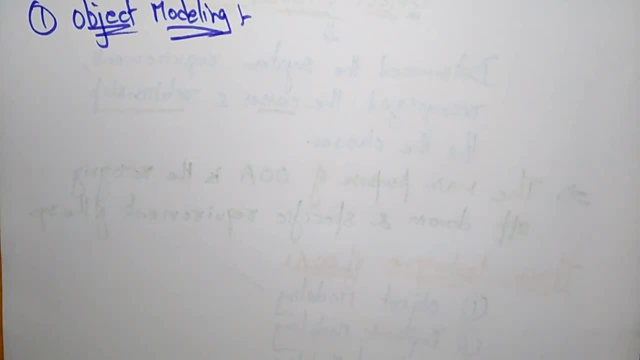 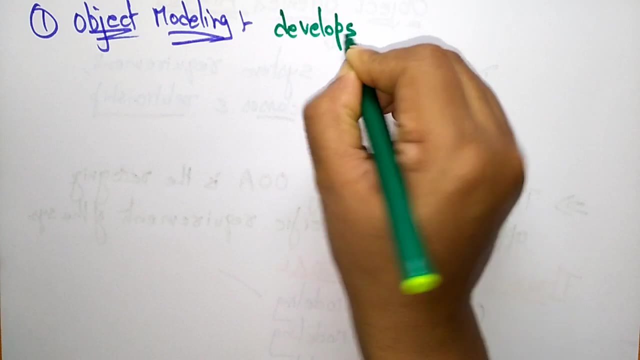 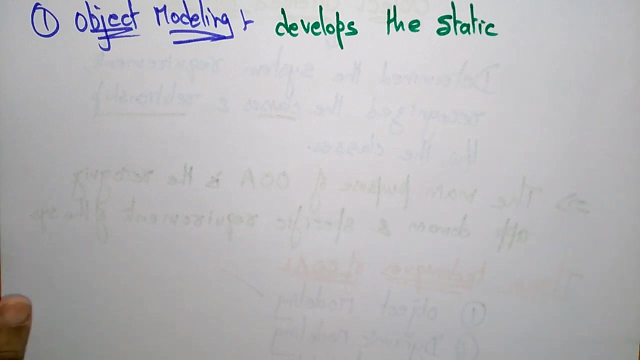 objects. objects are nothing but it's a instance of a class and it's a real-time entity. so this object modeling develops the, develops the static structure. so this point you have to be remember whenever you are saying that object modeling means object modeling is nothing but it is going. 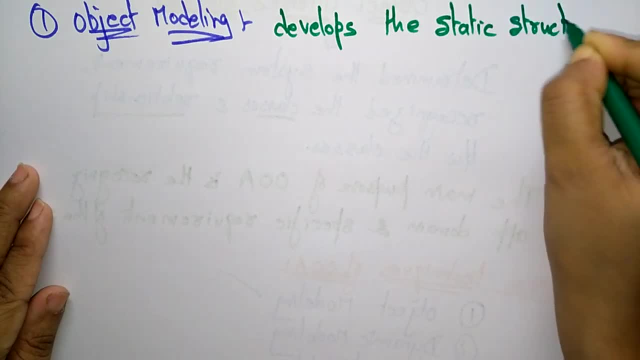 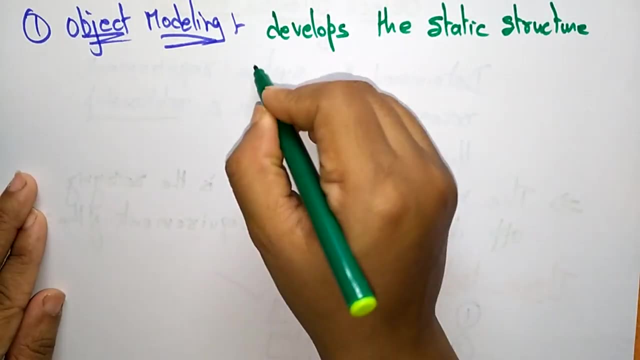 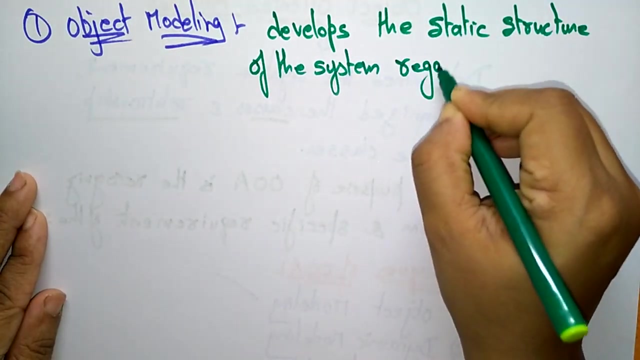 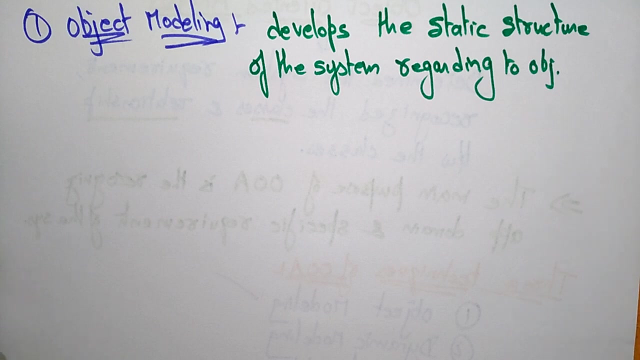 to develop the static structure. it's not a dynamic, only the static object. static objects. they are going to be created. so develop the static structure of the system. static structure of the system regarding to objects, so which is regarding to objects? regarding to objects, so, uh, the main in here: it recognize the objects first. it is going to. 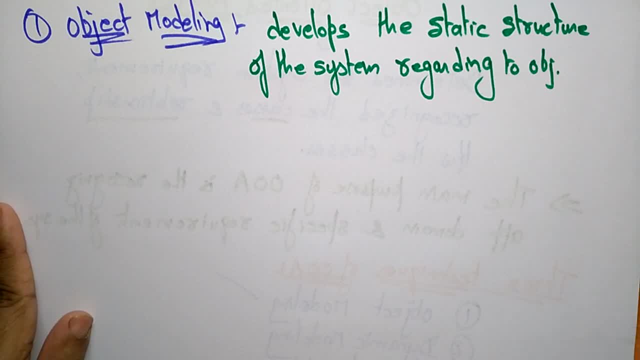 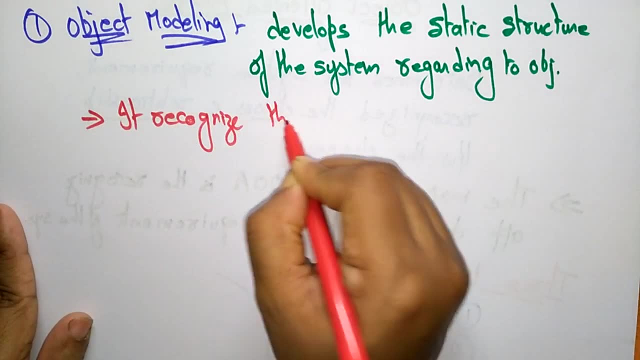 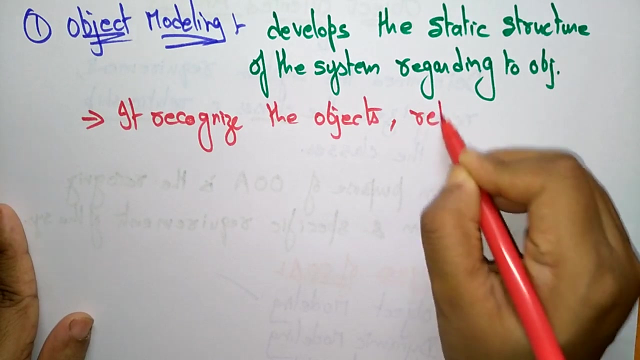 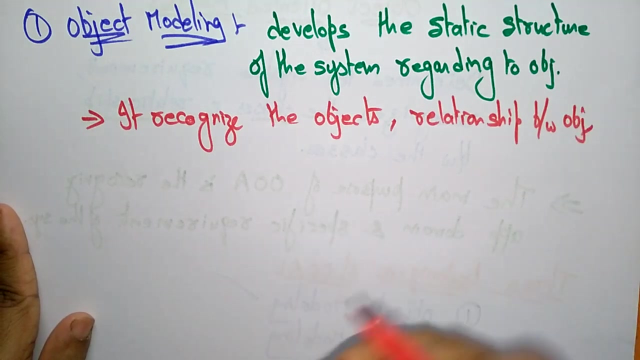 recognize that static structure of the system. uh, I mean I mean the objects which are related to the static. so first it recognize the recognize the objects that are present in the requirements, the objects, relationship between the objects, relationship between objects and the classes in which objects are grouped. 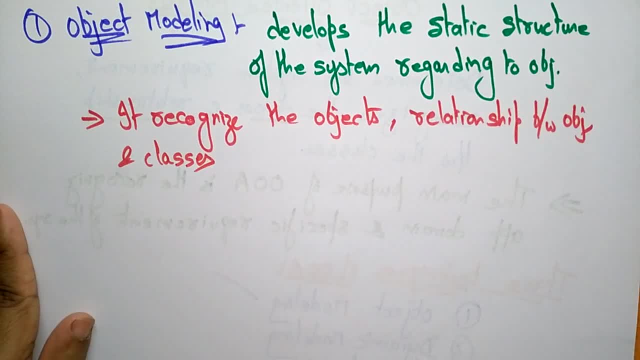 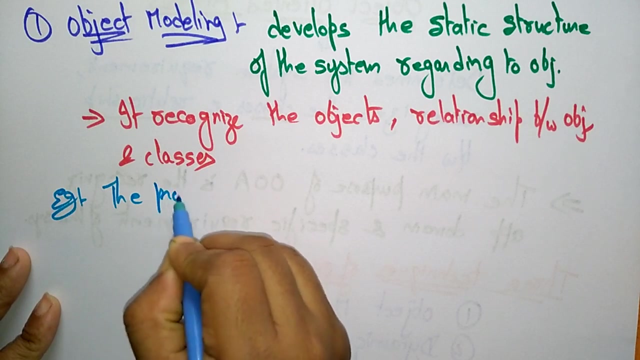 and classes in which the objects are grouped. so, uh, an object modeling is going to be so, and classes in which the objects are grouped. so how this will done. so let us see the process of object modeling. so here we take a look at the process of the object modeling process. 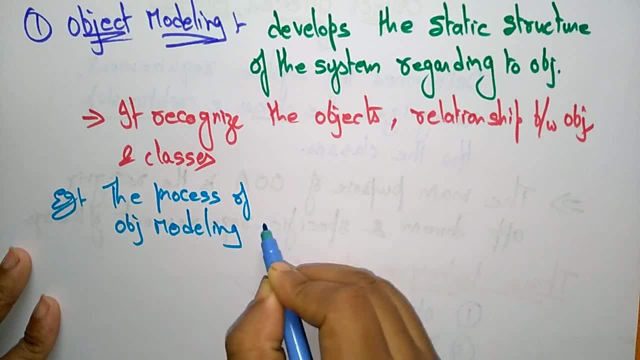 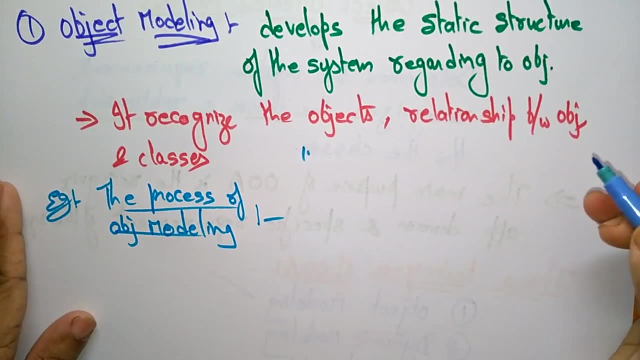 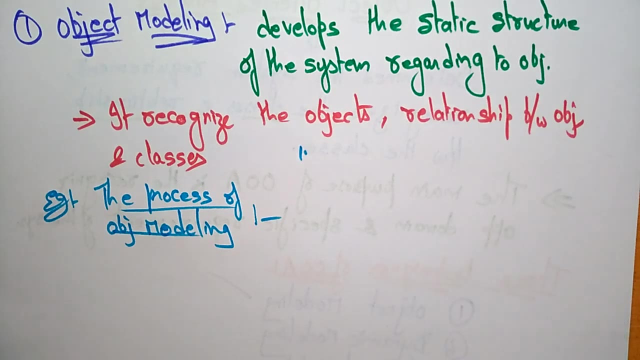 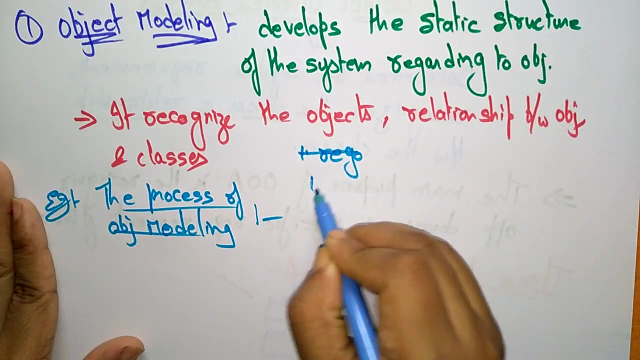 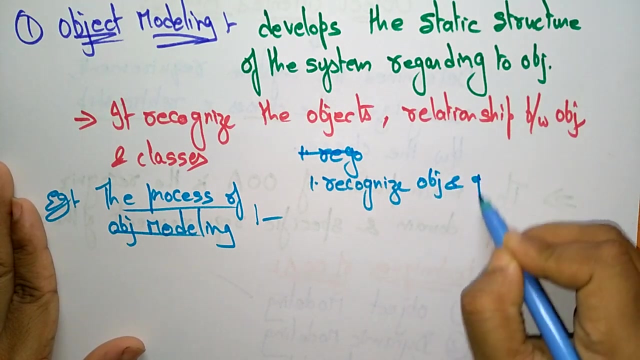 of the object modeling. so one of the public in the object modeling mind template obvious- can be used in the picture to explore the perception of the object modeling process. again, the spaces. So first is it recognize the object First? you have to. this object modeling is helpful to recognize the object and group into classes. That is the first thing: Recognize objects and group into classes and group into classes. 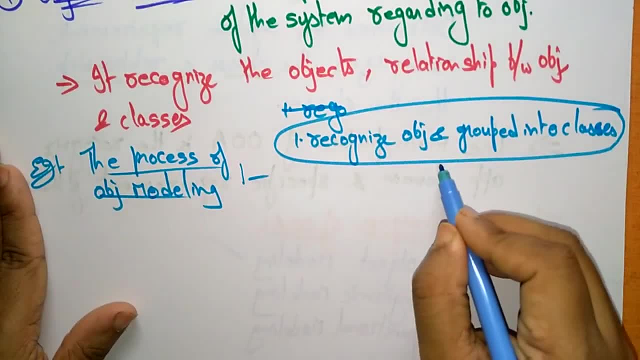 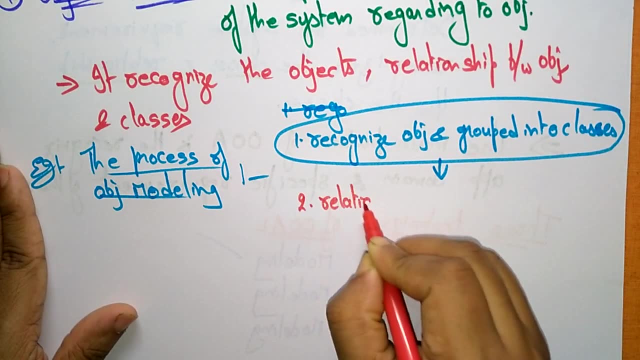 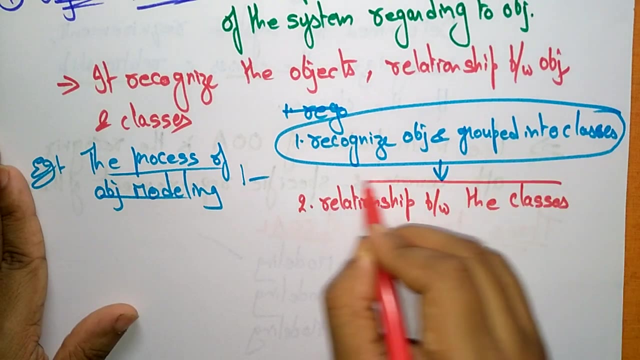 So, first, it is going to recognize the object and group into classes- Okay. next, Next, it recognize relationship between the classes, Relationship between the classes- Okay. and third, The third thing is it is going to the user object model diagram is generated. So, after recognizing the objects and they are grouped into classes, 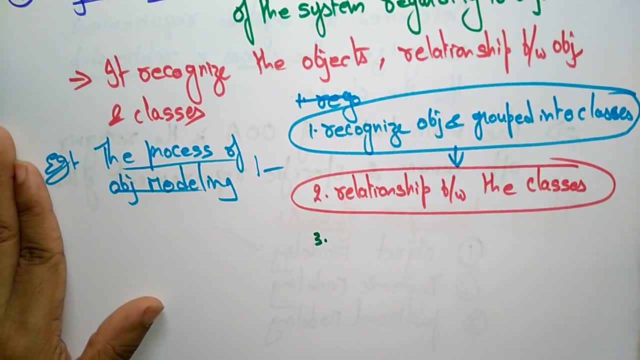 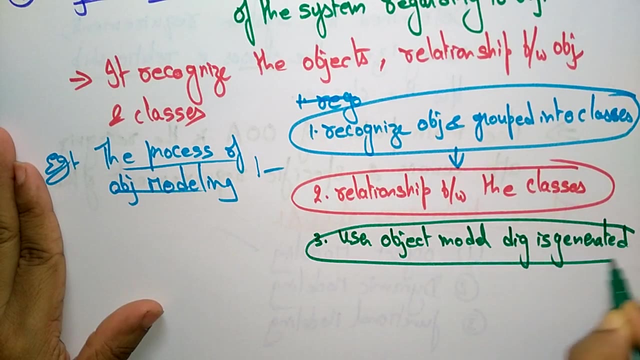 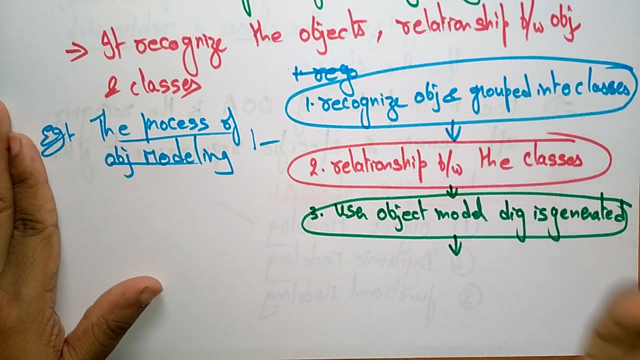 After that, the relationship is going to be established between the classes. Next is user object model diagram is generated. Next, user object diagram is going to be generated. Okay, After that we have to define the attributes of user object. So what are the attributes that are present? 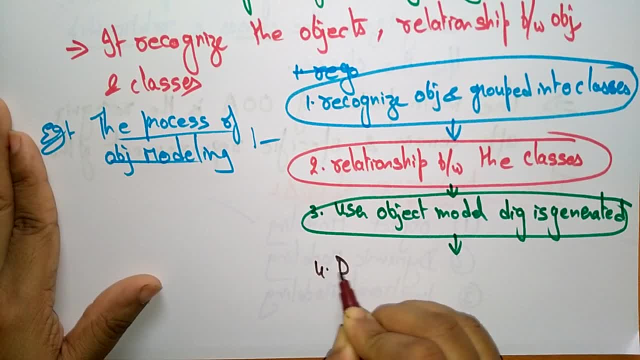 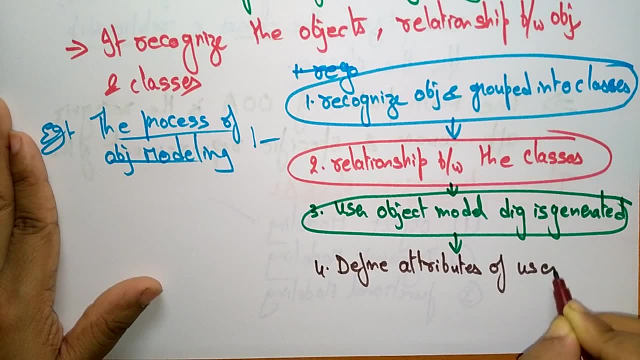 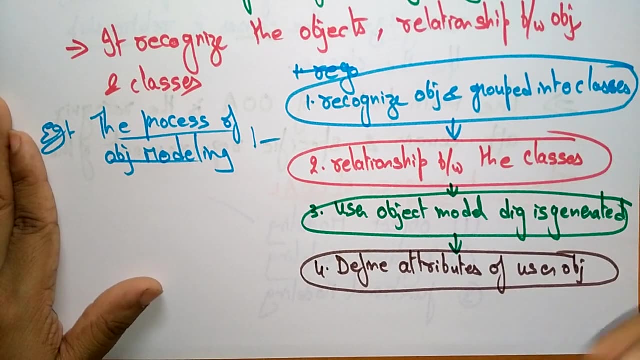 In this user object that we have to be defined, define, Define Attributes Of User object. So here just I'm explaining the process of object modeling. So if you take the object modeling, how the process, how the howit is going to be executed and next step,